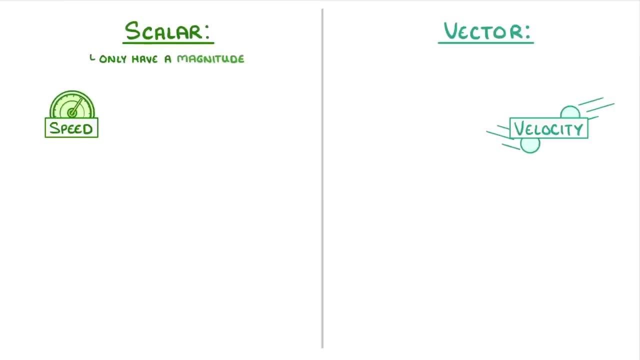 extent of something, whereas vector quantities have both a magnitude and a direction. So speed would be considered a scalar quantity because it only conveys magnitude. This might be a person running at 4 metres per second or a plane flying at 250 metres per second. 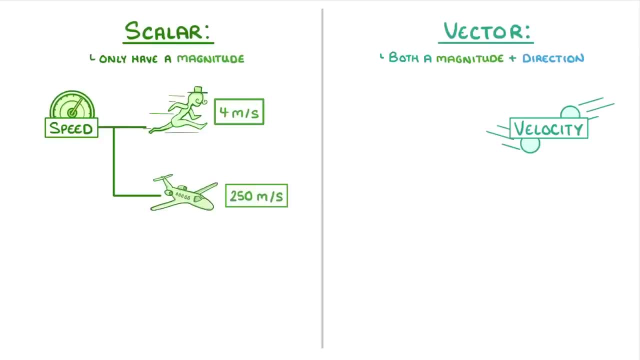 Velocity, on the other hand, is a vector because it also has direction, Like a person cycling 6 metres per second east or a train travelling backwards at 55 metres per second. It's really common in the exams to get speed and velocity confused. 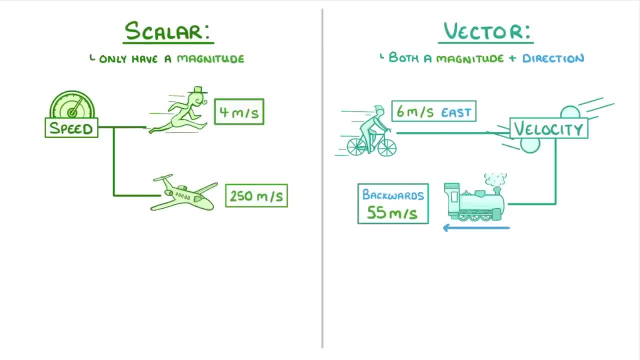 so just make sure you're completely sure about which one's which, and try not to get them mixed up. Another pair of quantities you need to know are distance and displacement. Distance is a scalar, As it only gives magnitude, like 10 metres or 40 miles. Displacement, though, is a vector. 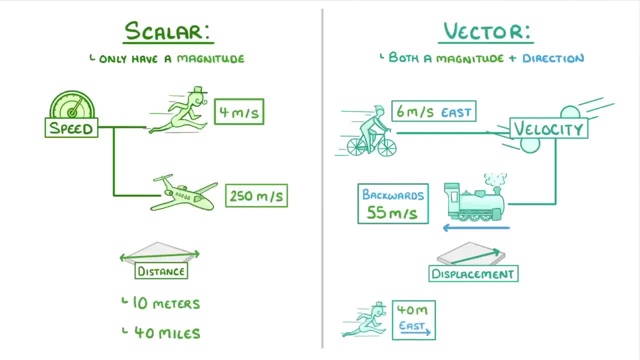 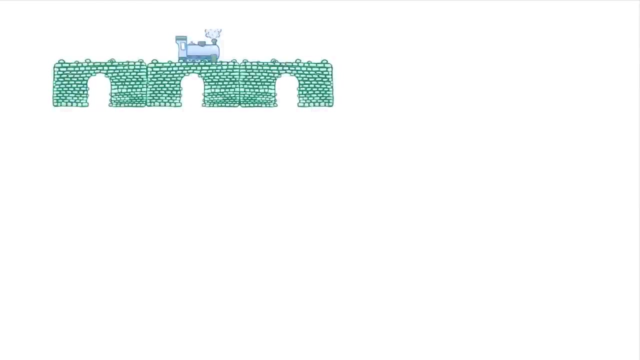 as it has direction as well, For example, a person running 40 metres east or a ball that falls 2 metres downwards. To help us understand this difference, let's imagine that we have a train travelling across a bridge. The bridge is 550 metres long. 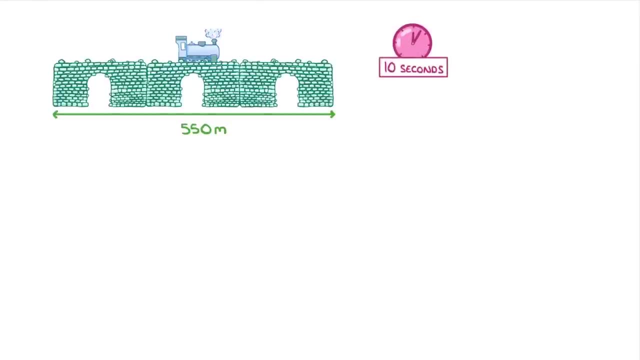 And it takes the train 10 seconds to cross it. To calculate the speed of the train, we need to take the distance it travelled and divide it by the time that it took. So 550 metres over 10 seconds, Which gives us the scalar quantity, or 55 metres per second. 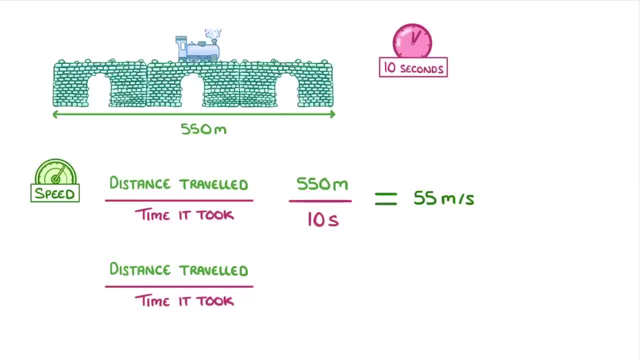 If we took this same equation but replaced the scalar quantity of distance and distance travelled with the vector quantity of displacement, we'd then be able to get the vector quantity of velocity. If we knew the direction that the train was travelling in, for example east, then instead 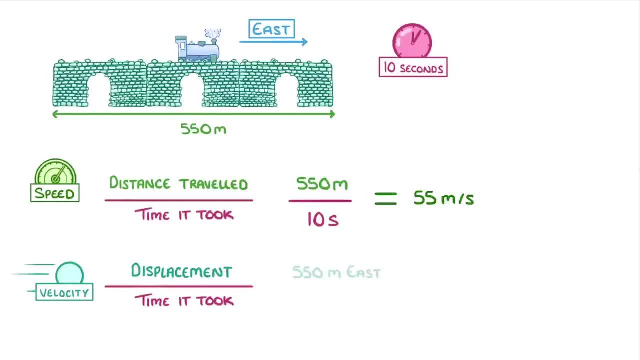 of writing the distance, we could write the displacement, which would be 550 metres east. The time would still be 10 seconds and the velocity would still have a value of 55, but the units of the velocity would be metres per second east rather than just metres per. 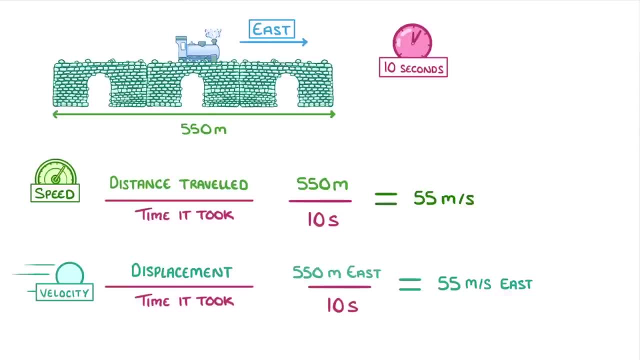 second, like we've got for speed. Now the symbol formulas for these two equations can be kind of confusing, because they use the letter S to represent different things. For velocity the S refers to the displacement, but in the speed equation the S stands for: 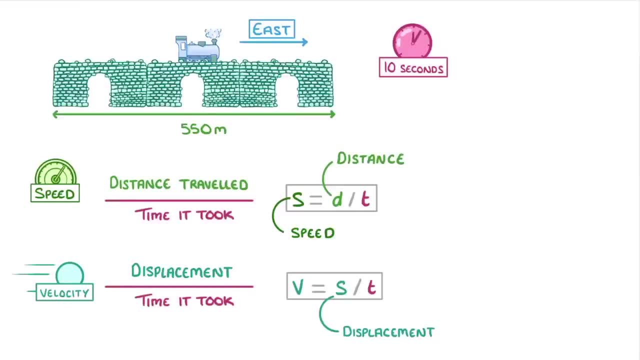 speed, The T is distance. In both cases, though, the T stands for time. In reality, people often use the velocity equation, regardless of whether they've actually got a direction or not. The benefit of using velocity is that you can have a negative velocity to represent. 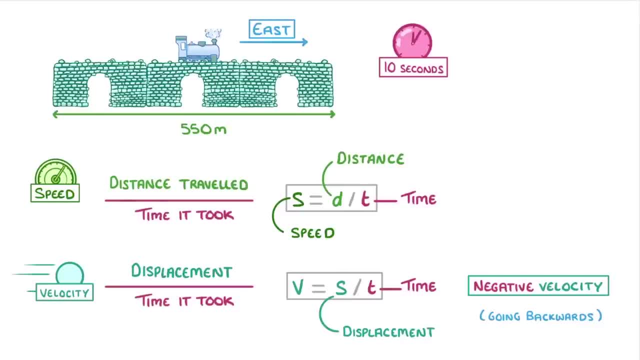 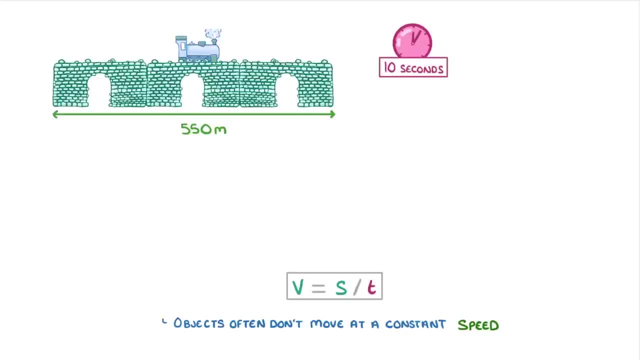 going backwards. Now, often objects don't actually move at a constant speed, But instead vary along their journey. We can still use this equation, but we need to divide the total distance, or displacement, by the total time that the journey took. 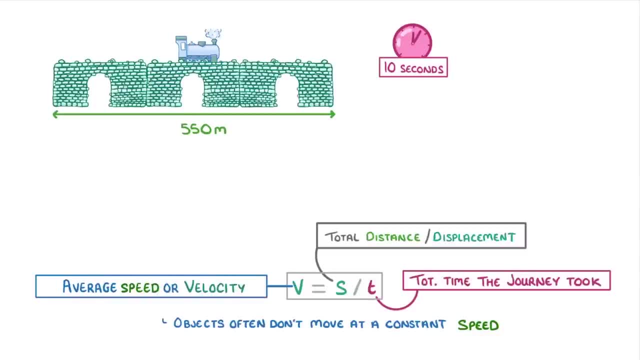 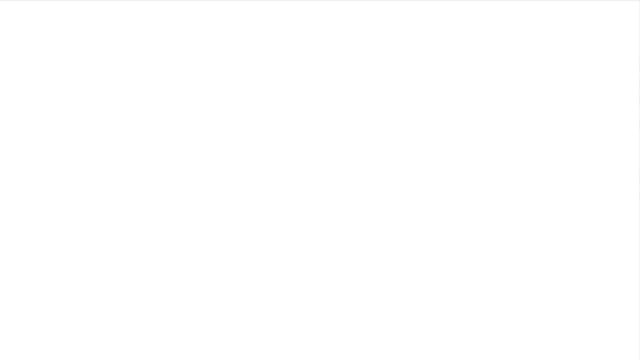 And the value that we calculate will then be the average speed or average velocity. To give you an idea of real life speeds in metres per second, people walk at about 1.5mps, run at about 3mps and cycle at about 6mps. 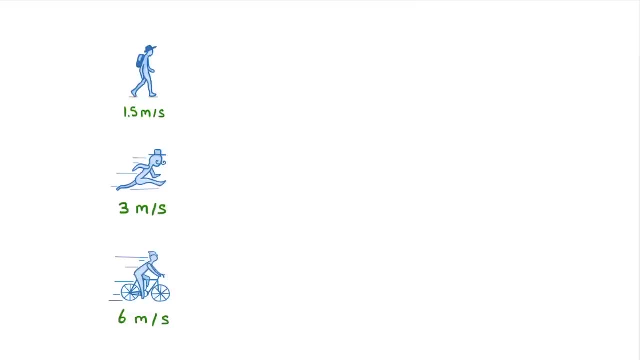 All of these numbers do, of course, vary a lot, though, depending on the age and health of the individual and how much effort they're putting in at the time. Then, for vehicles, a car on the main road might travel around 25mps, while a fast train. 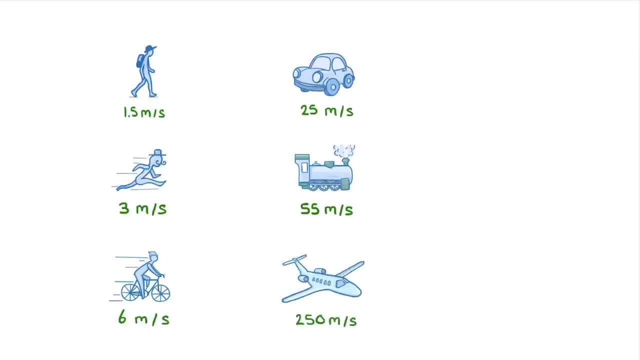 could travel 55mps And planes can travel around 55mps. So that's the difference. It's not only the speed of objects that varies, though. As we'll see in a later video, sound waves travel at 330mps when they're in air, which? 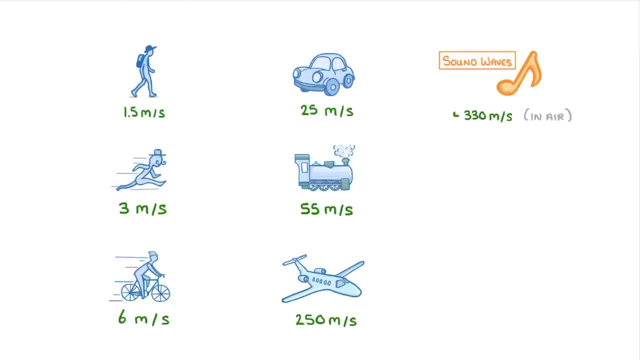 is a figure you need to remember. But when they're travelling through different mediums, like water, their speed changes. A more relatable example is the wind, Which is just the natural movements of air. This can vary from almost 0mps on a still day to faster than a speeding train on a 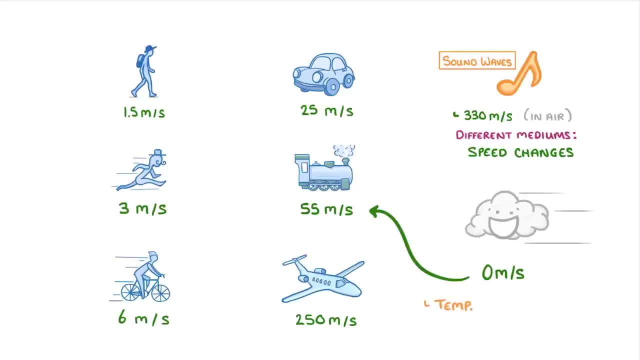 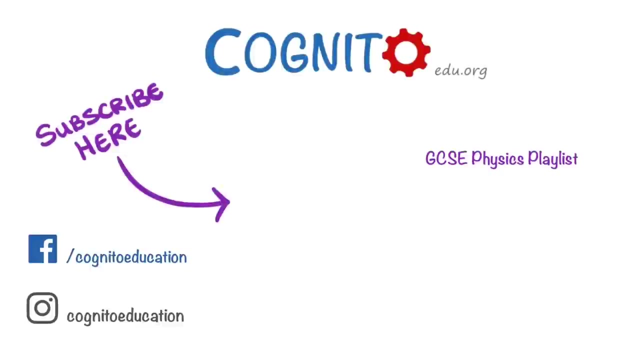 windy day And can be affected by things like temperature, atmospheric pressure and these structures it's travelling past like buildings or mountains. Anyways, that's everything for this video, So hope you enjoyed it and we'll see you next time. 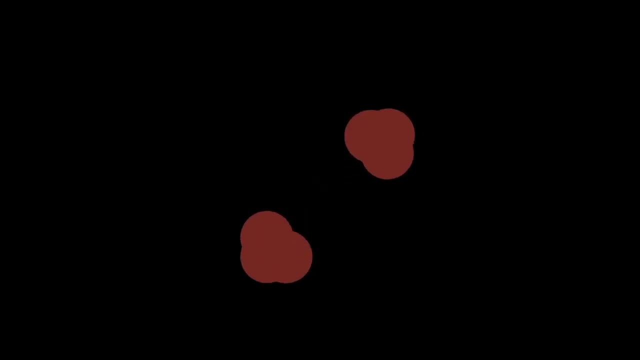 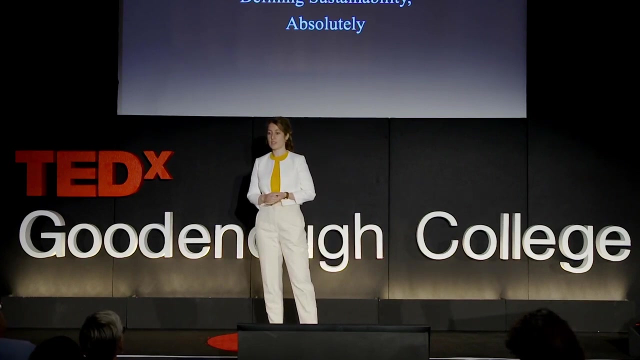 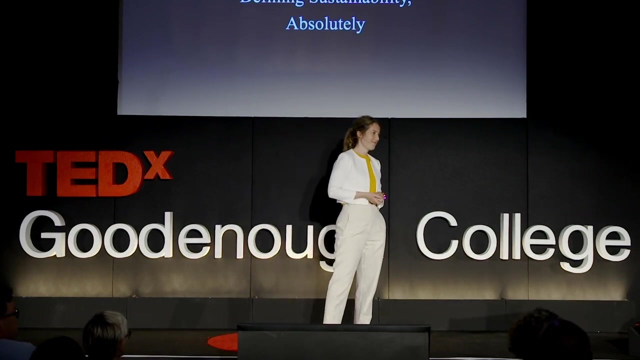 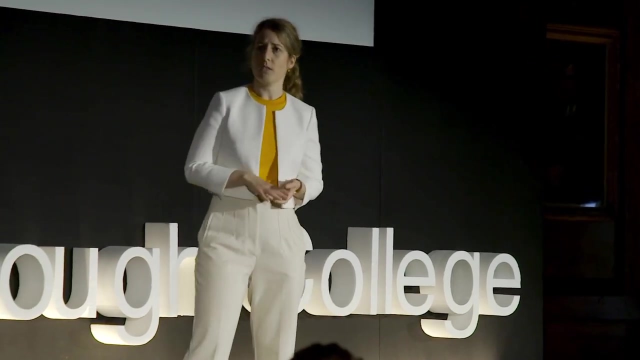 How many times this week have you heard something referred to as sustainable? It could have been sustainable cotton, Sustainable coffee, Sustainable single-use cutlery. I've heard that. I heard another good one: Sustainable coal. I think the best one I've heard yet. 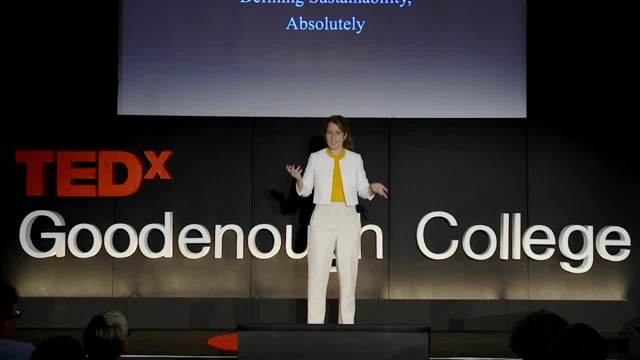 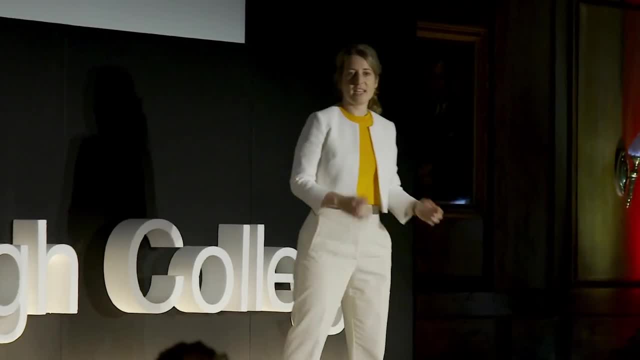 is sustainable. airship, hotel. What is that? even I don't know. Yeah, People use the word sustainability to mean a lot of things, And the vagueness of the word can be put into two different groups: One of focus and one of non-focus. 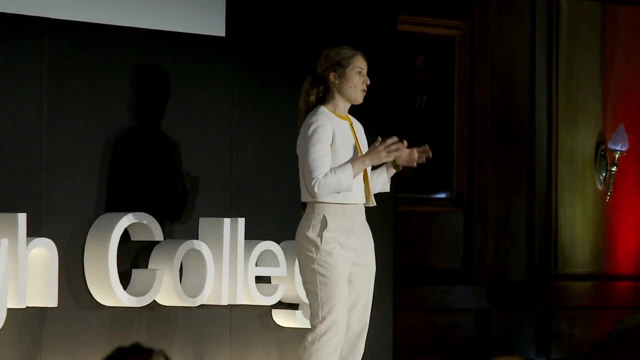 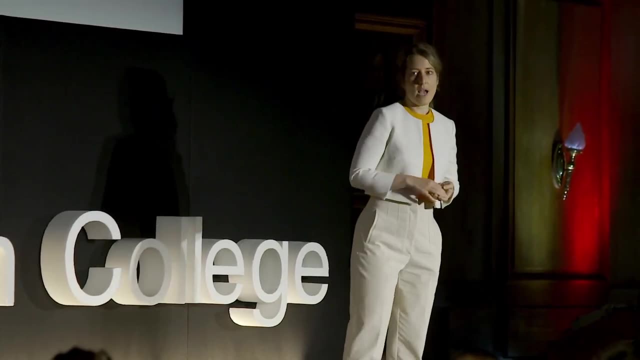 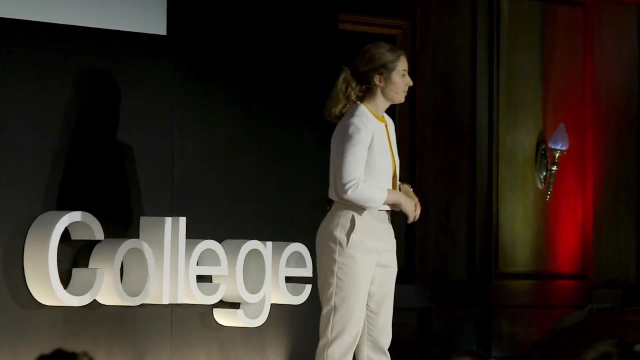 The focus problem arises when we say something is sustainable but we're only addressing sustainability in one aspect. Take sustainable cotton. Usually, when you dig into it, sustainable cotton is organic cotton, And organic cotton is great if you want to reduce the amount. of pesticides you use and the toxic pollutants that you emit into the environment. But organic farming is also associated with lower yields, which means we need to use more water, We need to use more land And there are higher associated carbon emissions. Now the numbers. 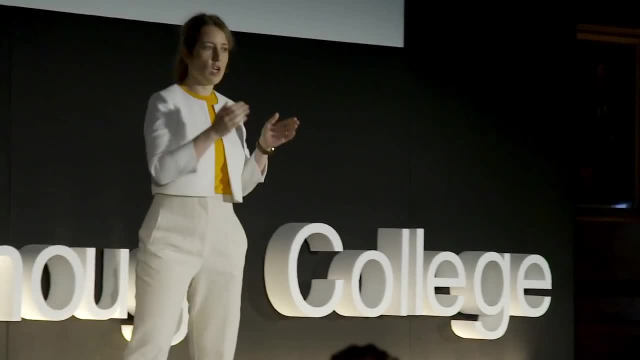 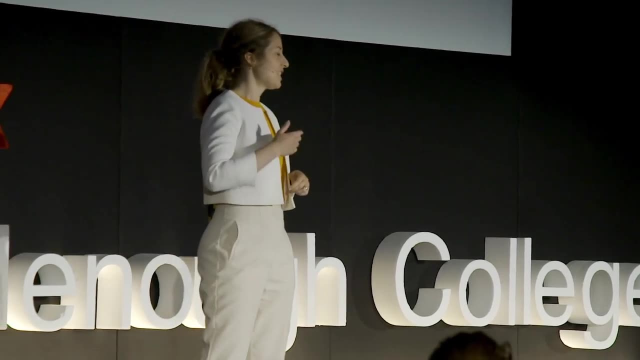 problem arises when we say something is sustainable, but what we really mean is it's just more sustainable than something else. Take a nice hot cappuccino, maybe one you had this morning. If you had a cow milk cappuccino this morning, you might have noticed that it was a bit cold. If you.